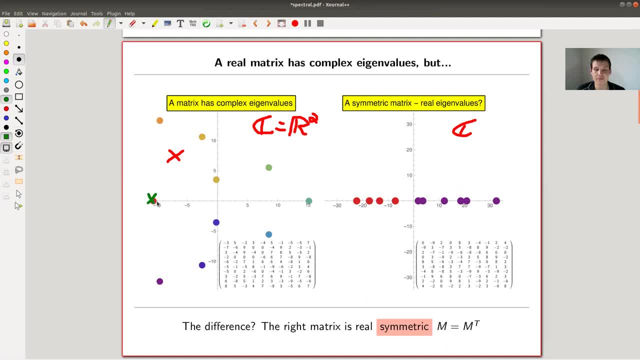 So you can see here, for example, for the matrix at the bottom, you have two real eigenvalues and the rest are really imaginary eigenvalues. they're not real And you don't. you shouldn't look too much at the matrix here at the bottom. It's a matrix I created using random integers. 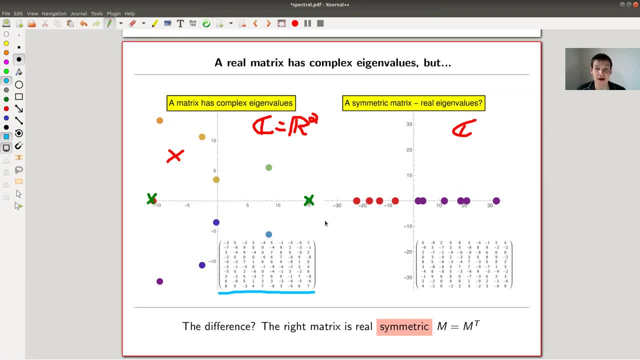 And you don't. you shouldn't look too much at the matrix here at the bottom. It's a matrix I created using random integers, So it's just at least 9 eigenvalues. This is basic linear algebra of the problems, And then theoretically we just have to take ten 지역s, from minus nine to nine. 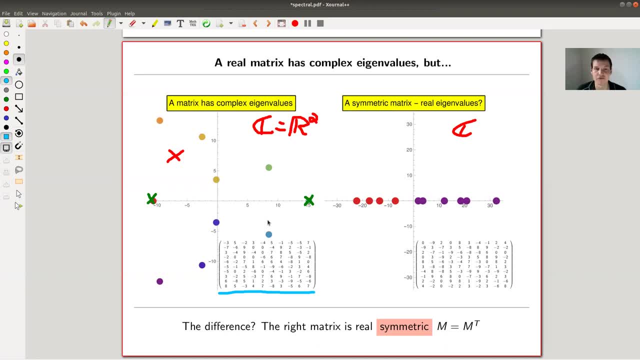 Ten by 10 matrix. So if you just plot to the spectrum of the ten by ten matrix, just kind of random entries, Of course they will be complex eigenvalues, Just just as I said it again, what you need do is you would need to calculate a characterization polynomial and to check what its roots are, And it's super unlikely that you will end up with 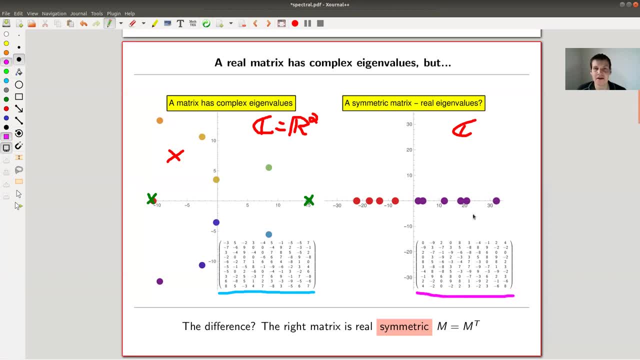 did the following. i also constructed the random matrix, but it's not completely random. so this matrix, actually um, is symmetric, which just means it's its own transpose. in other words, along the diagonal, you allow whatever you want, and whatever is upstairs is reflected downstairs. this is just. 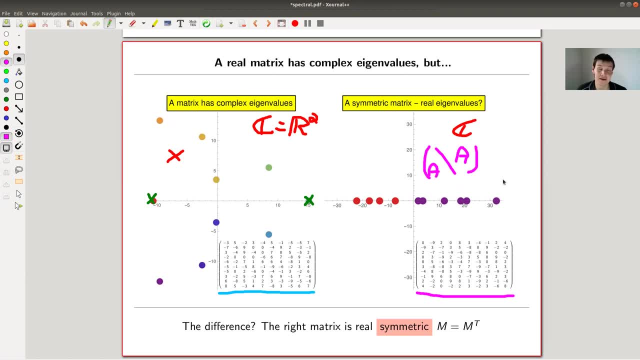 symmetric uh, otherwise it's again basically random integer entries from my uh, from this, from minus nine to nine, and well, then you plot the spectrum and you will see that everything here just is real. so all eigenvalues are real and this just can't be a coincidence anymore. 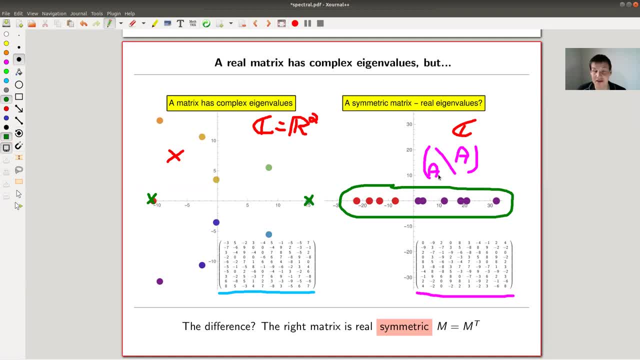 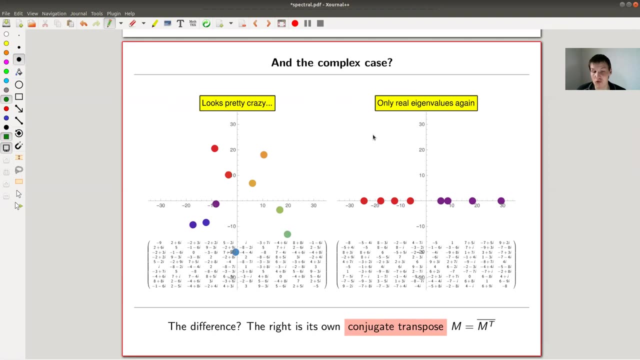 because, well, you're just constructed, uh, you just looked at the eigenvalues of a basically random matrix, so the only obstruction you had is that it's symmetric. that's already a good hint that something is going on. then you might play a little bit more, like down here. i basically played the same trick. i have two matrices, a red one, 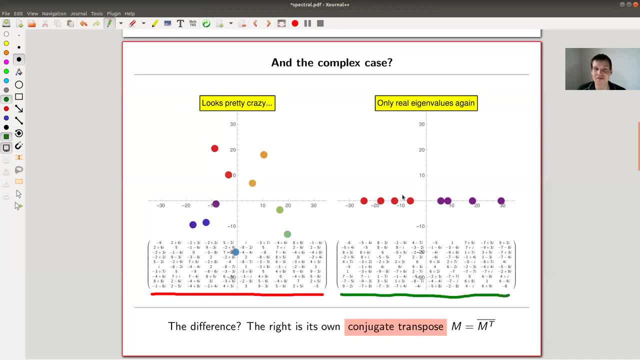 and a green one. and now the entries are even worse. they are kind of random complex numbers and there's just just no way. there's just no way that you don't end up with some reasonably crazy looking pattern, again the same same thing. you have c here or r2, whatever you want. 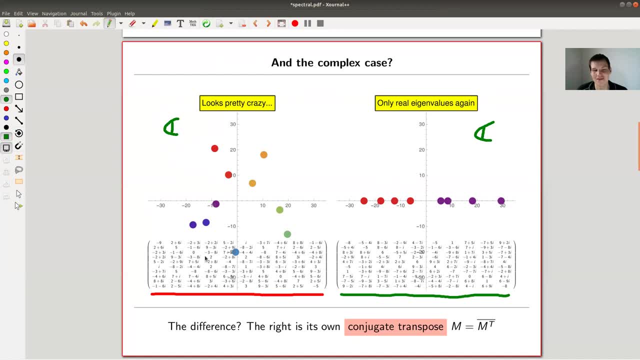 and you plot the eigenvalues and it looks pretty crazy. on the right hand side i have this funny condition which is called the complex transpose. so actually the matrix is as before, is something on the diagonal, just real entries on the diagonal, which comes from the condition of being its own complex. 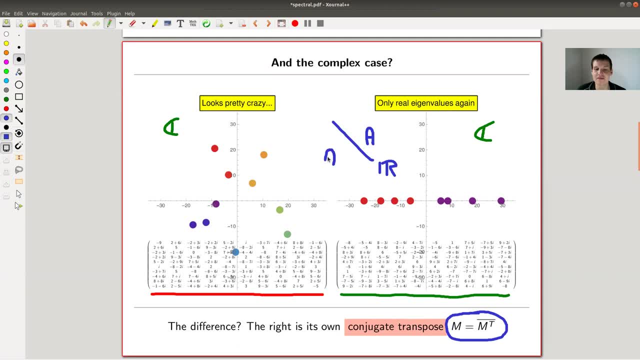 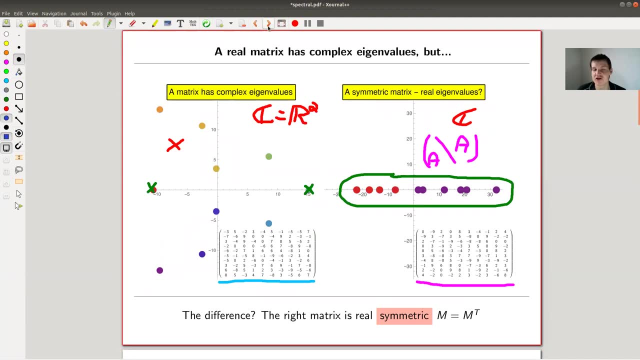 transpose some matrix upstairs here and not quite the same matrix downstairs here. but you need to take the complex quantity. so, in contrast to the real case where you just have aa, which i've called symmetric, in the complex case you have a and a bar. so taking the complex quantity, 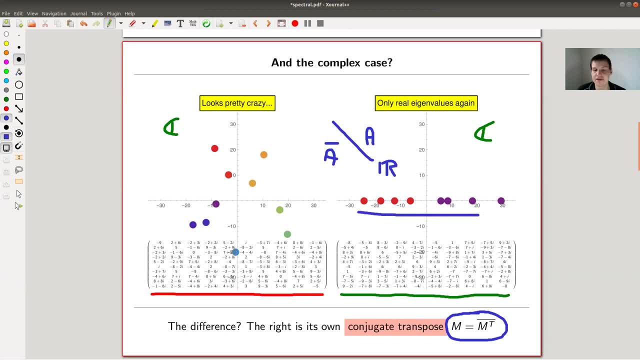 you create a random matrix- again the green one- and, as you can see, the green one has really nice eigenvalues in the sense that they're all real. i mean this just can't go. can't be a coincidence, right? you have a 10 by 10 matrix. basically your entries are real. 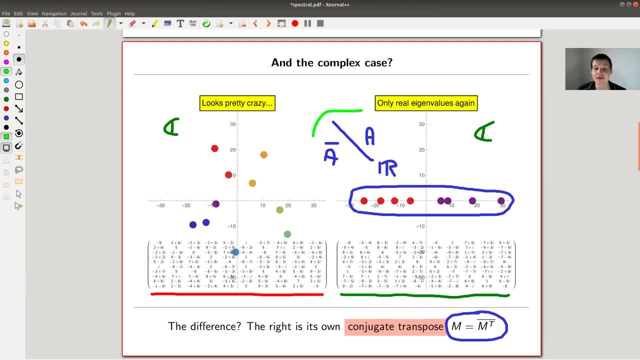 the only obstruction you added is exactly this one here, right? so this can't be a coincidence, and this will be exactly the statement of the spectrum field. spectrum theorem is actually a little bit better, so let's look at that. um, so here i have. well, let's go back to the real case. so we 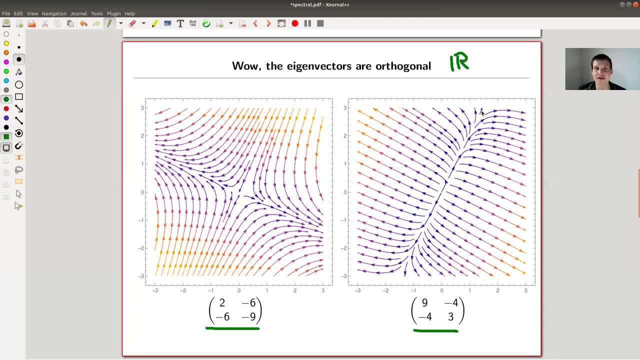 are back to the real case. they're subject similar in the complex case. i just can't make such nice plots anymore. so i have two symmetric matrices- uh m and m, prime, whatever- and they're certainly symmetric. as you can see, there's something on the diagonal and you have a symmetry by the matrix. 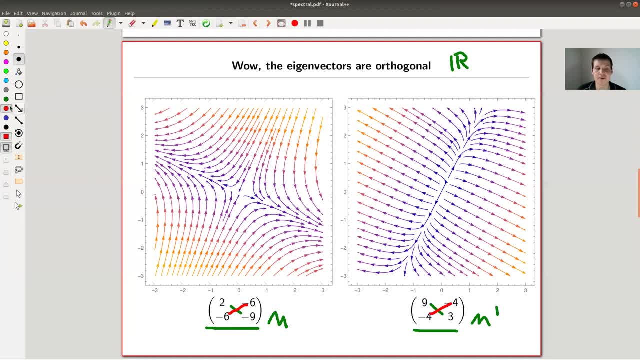 by flipping along the diagonal and i just plotted basically, um, their action on on this is r2 and this is, of course, also r2. i basically plotted the action on r2 and as you, so here are the eigen values. you can the eigenvectors, you can see the eigenvectors. so here's an eigenvector, as you can. 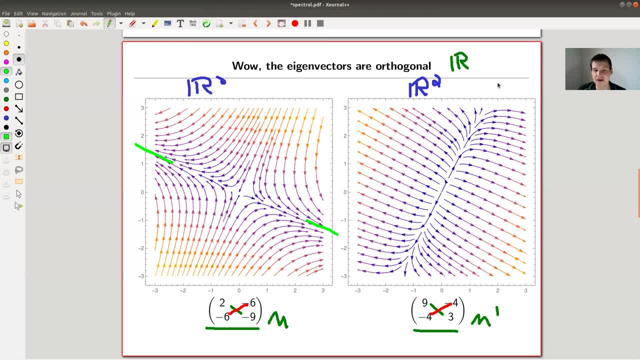 see a green one and similarly, here is an eigenvector, which is something that's fixed right. so in this picture it's it's always easy to see something that's fixed. there's also a blue one which is roughly here, a blue one, a red one which is roughly here. it's a bit harder to see, but it's. 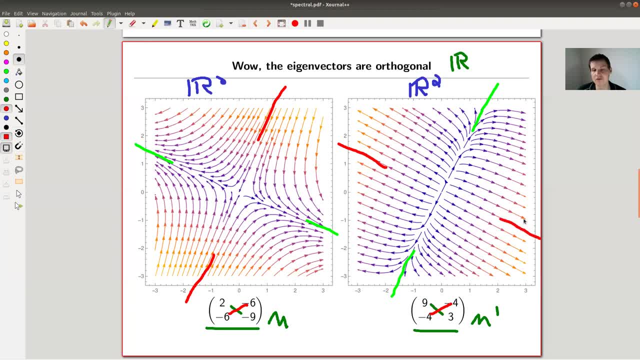 roughly here. uh, so along those lines, you have the eigenvectors, you have two of them and you not just have two of them, which is really good, because it basically means it should be diagonalizable to linear, independent and eigenvectors, um, but they are also certainly orthogonal to one another, which is very surprising. 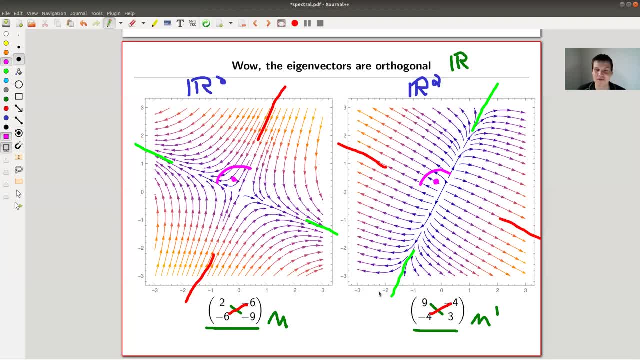 because i basically again took now two by two matrices, because otherwise i would need to plot you an art out of the ten and i don't know how to do that. but anyway, they're basically random entries, since the only obstruction i had is i wanted to be them to be similar, symmetric. 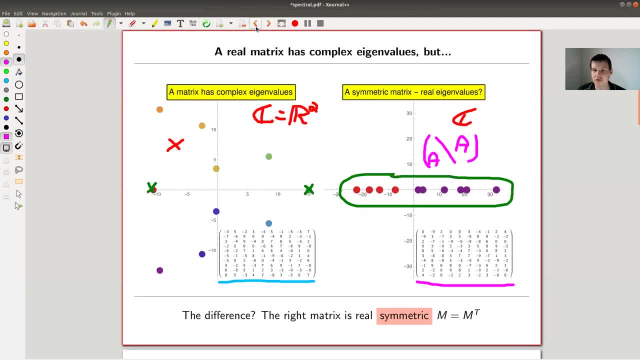 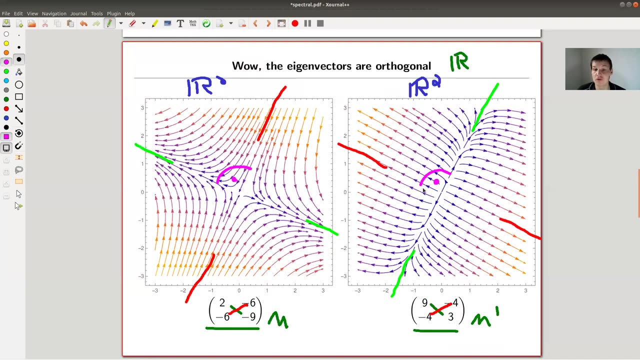 so what have you seen? okay, we have seen. um, so let's ignore the complex case for the for a moment. it's a similar, but you need to take the complex conjugate. so if you have a real matrix which is symmetric, you get real eigenvalues and apparently you also get orthogonal eigenvectors, and that's. 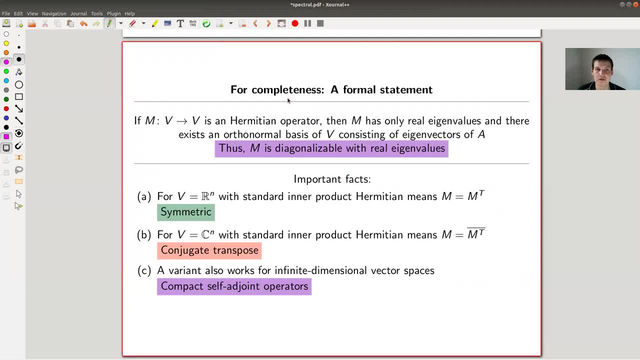 exactly what the um, what the theorem says, the spectral theorem. so if you have an image in operator which, which is, is just symmetric, in the case you have r to the n, don't worry too much about it because it's just a common terminology and it's um conjugate transpose in case um. 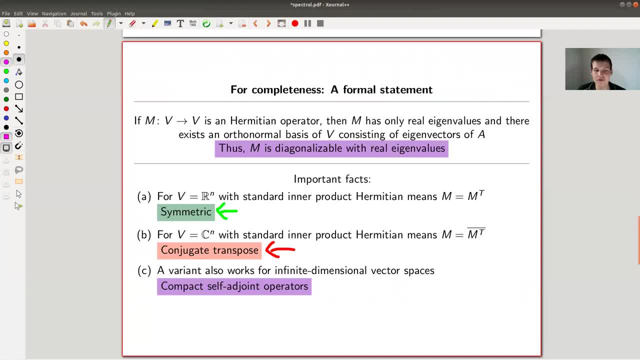 you are c to the n. and then the point is: well, first of all, m is diagonalizable, it's only real entries, but not just that. so all eigenvalues are real and you have an orthogonal basis of v, which is actually orthonormal. so you can't see in these pictures that they are actually orthonormal. but you have to, you have to. 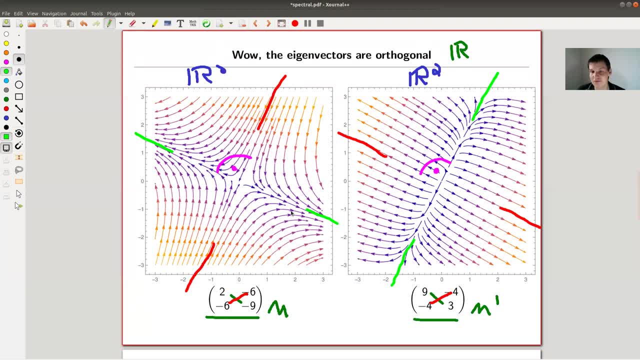 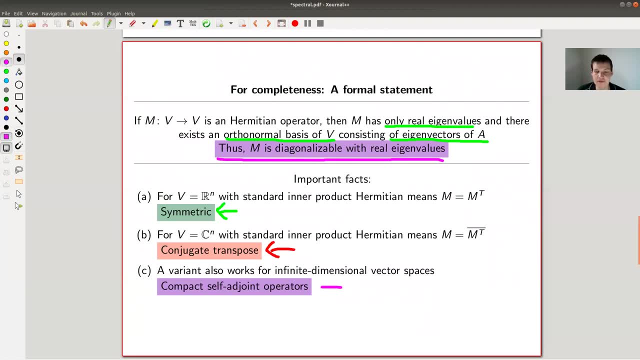 you have to normalize them anyway. um, anyway, and this also generalizes to infinite dimensional spaces. i'm not going to do that, but anyway. so this is a really, really basic and powerful theorem of linear algebra which, as i said, generalizes, like to infinite dimensional vector spaces. you 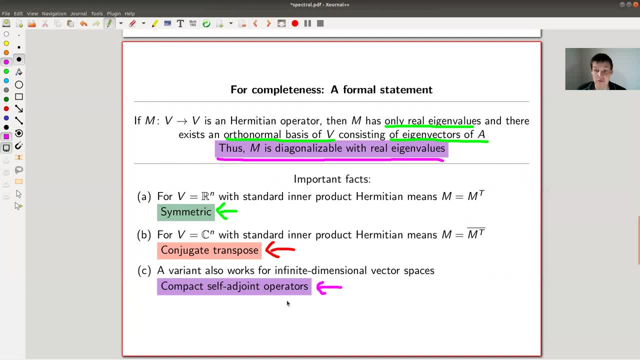 will see it in the next slide. so this is a really, really basic and powerful theorem of linear algebra and it's basically what functional analysis is and it's a really, really easy statement. it's: you look at the matrix, it's symmetric or or whatever this hamitian property. 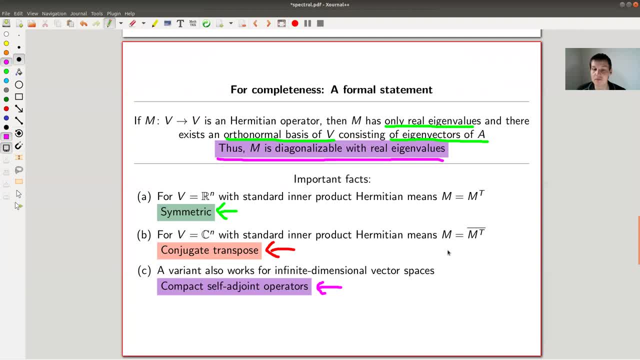 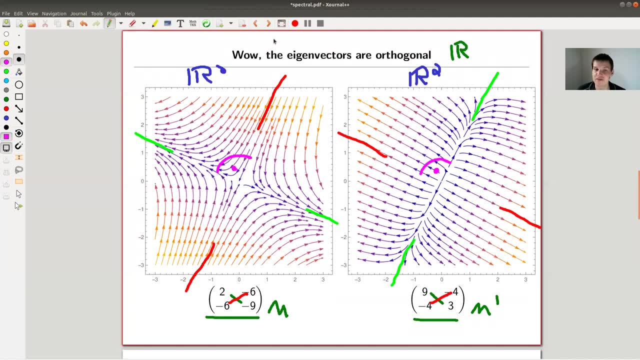 and all eigenvectors are real, eigenvalues are real and eigenvectors form an orthonormal basis, which is- which is pretty, pretty amazing, because why should any kind of real symmetric matrix have any kind of real eigenvectors? because it's just, it's just a very simple formula. 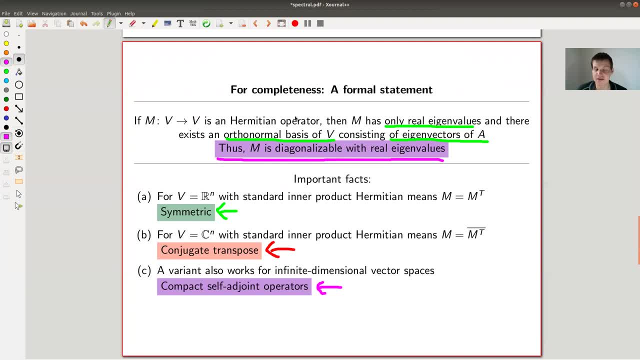 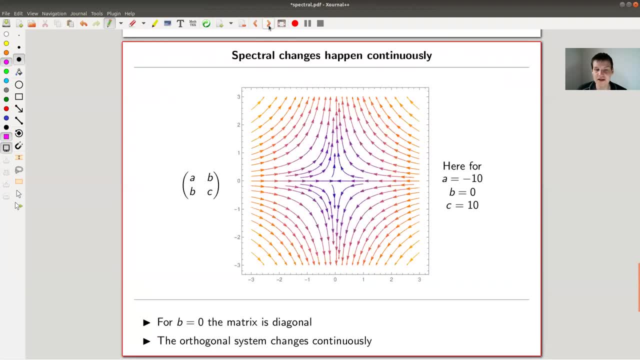 and you can't satisfy that um. so that's a spectral theorem. it tells you something about the spectrum of hamitian in general, or let's say symmetric matrices, and actually it's pretty nice, um, because everything kind of happens continuously. so here is a plot of a symmetric matrix which i 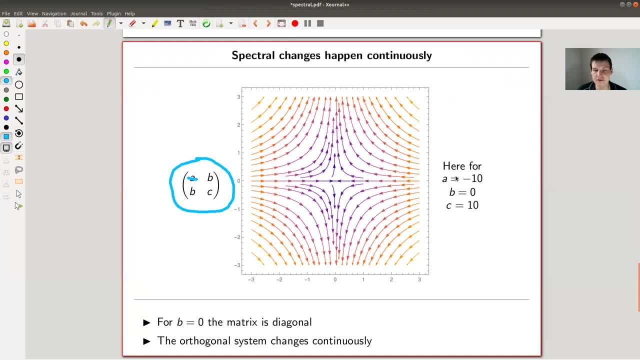 will vary in a second in the video. so i have three entries. i have an a entry, a is minus 10. i have a b entry and in this picture here b is 0 and i have a c entry and c is 10.. so b equals 0, means this is a diagonal matrix and you should see. 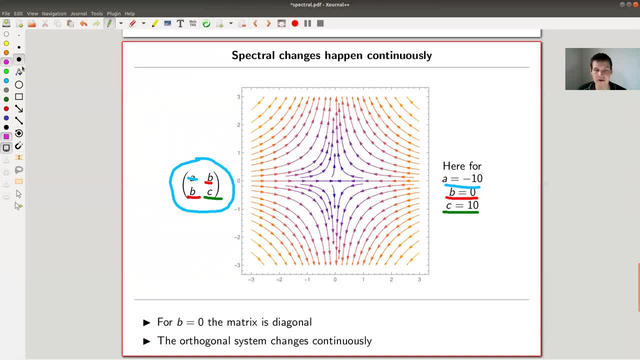 um the well, uh, the coordinate axis is eigenvectors and yes, here you go. so this is one eigen axis, another one, and i will now vary this picture continuously in um the entries a, b, c, and you will see that that every it's really beautiful. so you will see that, um, the angles always be kind of preserved, not the. 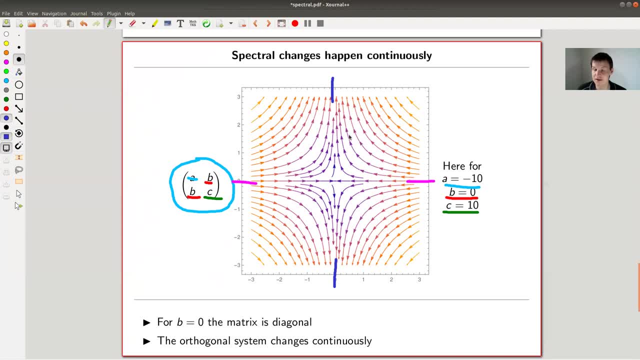 angle, so it you always uh, have those two eigen axes which are in 90 degrees to one another, and as soon as you hit the b equals zero, you will exactly end up with such a picture like this, where the eigenvectors are actually the x and y axes. it's the picture. 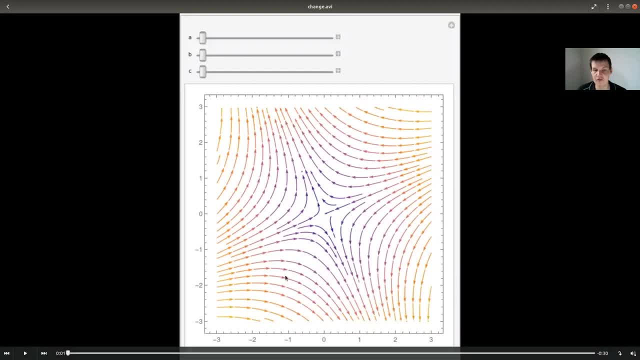 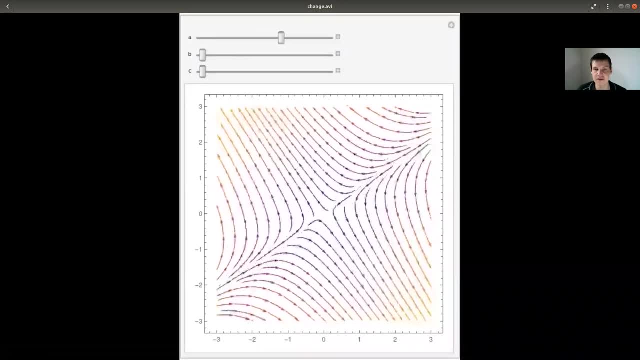 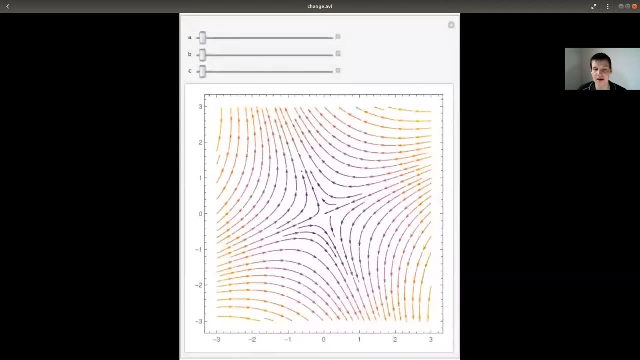 okay, here we go. so we have, as i said, i have a, b, c, and never vary them now in this video. so let's, let's watch it so, as you can see, it varies very continuously and you can really see the coordinate axis moving, the eigen axis. if you vary b at one point, it will cross x, y.